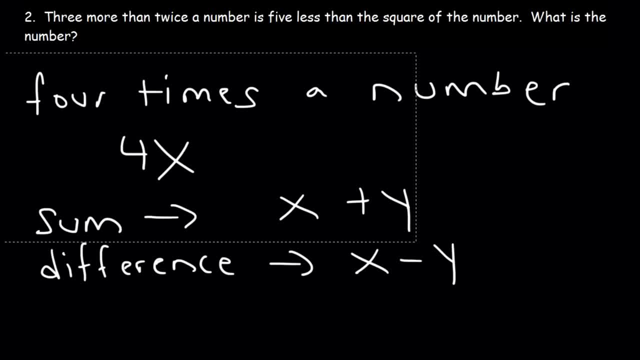 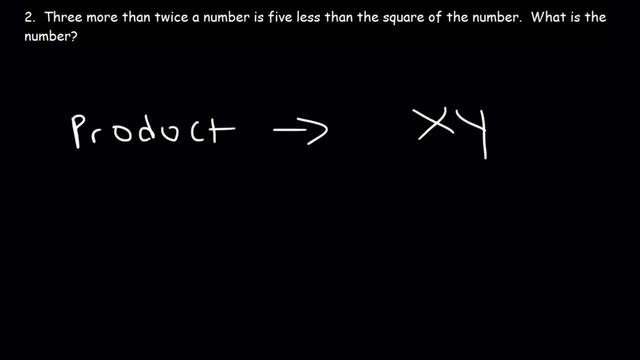 That would be x minus y. Now what about the product of two numbers? The product of two numbers is associated with multiplication. That's x times y. Let's say, if you hear the word 5 more than a number, What's 5 more than a number? 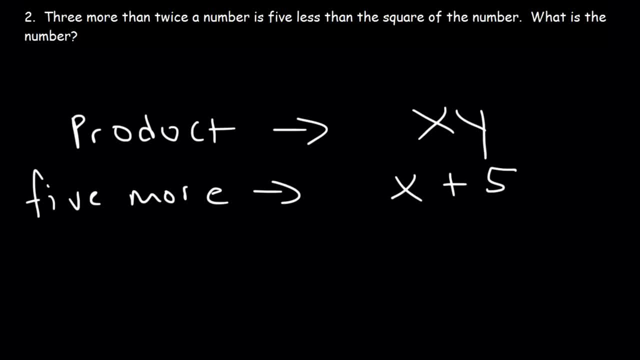 This would be the number plus 5, or 5 plus x. Let's say, if you hear the word 4 less than a number- Now this one- you need to be careful. if you hear this expression. 4 less than a number is not 4 minus x, it's x minus 4.. 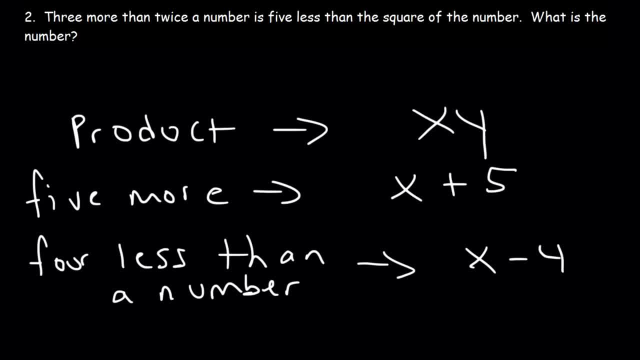 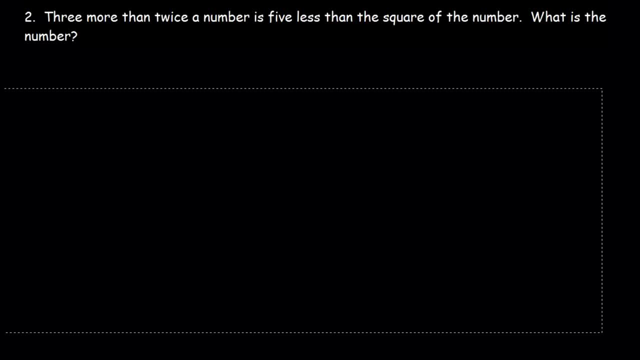 So the 4 comes after, Even though in the sentence the 4 is written first. So watch out for that one. Now, what about the square of a number? If you hear the word square of a number, that's basically x squared. 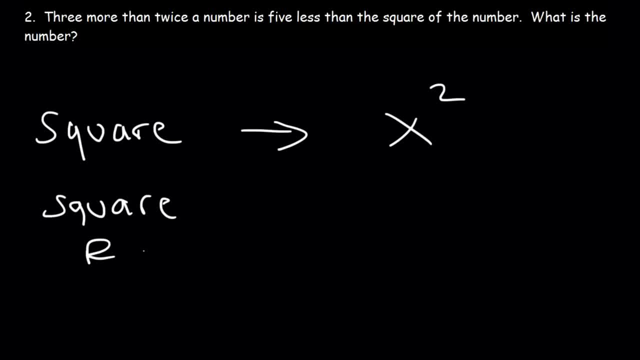 If you hear the square root of a number, then you're dealing with the square root of x. Now, what about this one? What's 7 times the difference of two numbers? 7 times the difference of two numbers? We know the difference of two numbers is x minus y. 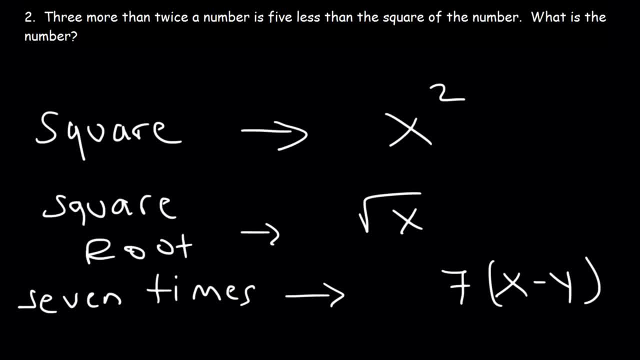 And then whatever that difference is is multiplied by 7.. So the 7 is in front of the x minus y, within the parentheses. The 7 is outside the parentheses but the x minus y is within it. So those are some common expressions that you need to be familiar with. 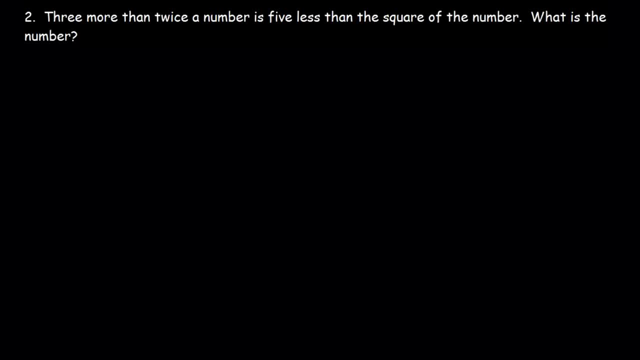 Number 2. Number 2.. 3 more than twice a number is 5 less than the square of the number. What is the number? So go ahead and pause the video. Try this problem, See if you can figure it out. 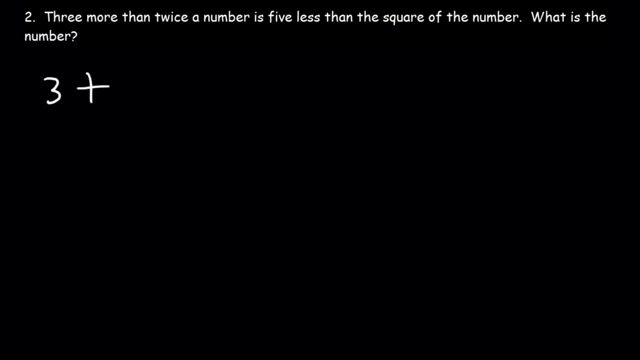 So 3 more, that's going to be 3 plus, and then twice a number that's 2 times x, And then we have that word is, which is associated with equal, 5 less than the square of the number. 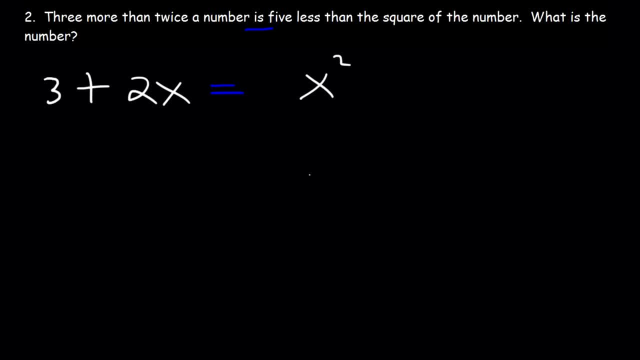 The square of the number is x squared. Now we don't want to write 5 minus x squared. The 5 comes after. It's going to be x squared minus 5, so don't make that mistake. So our goal is to find the value of x. 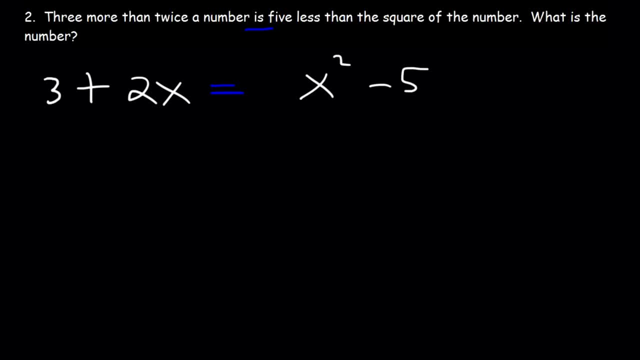 How can we do so? On the right side, we have the variable squared. On the left, it's not squared. What we have is a quadratic formula problem or a quadratic expression. We can factor the equation or we can use the quadratic expression. 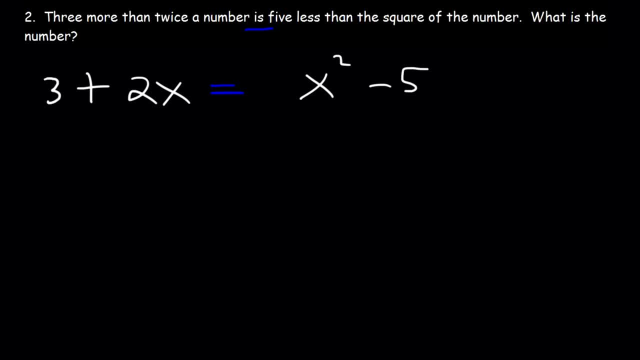 or we can use the quadratic formula to find the value of x. Let's move everything from the left side to the right side, So let's subtract both sides by 2x and by 3 at the same time, So on the left side we have a 0. 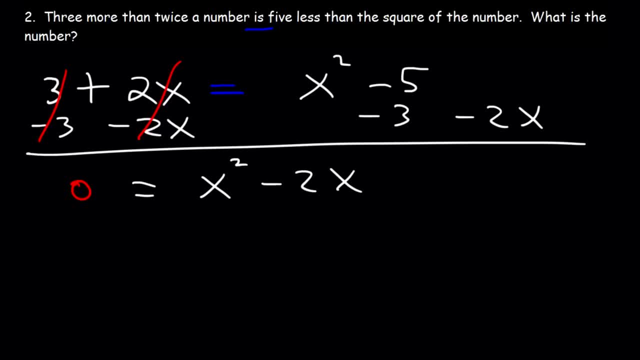 On the right, it's going to be x squared minus 2x. Negative 5 minus 3 is negative 8.. What two numbers multiply to negative 8, but add to the middle coefficient of negative 2? This is going to be negative 4 and positive 2.. 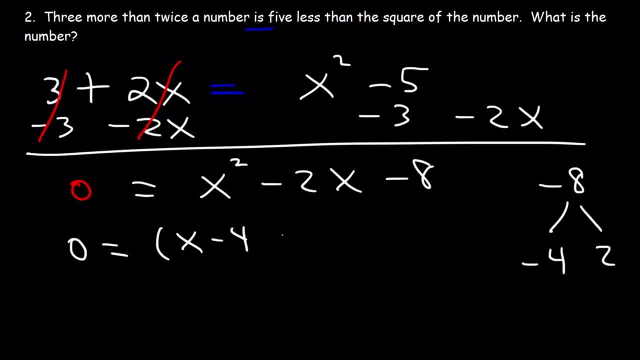 So to factor it, it's x minus 4 times x plus 2.. At this point we need to set x minus 4 equal to 0, and x plus 2 equal to 0. So if we add 4 to both sides, we can see that x is equal to 4.. 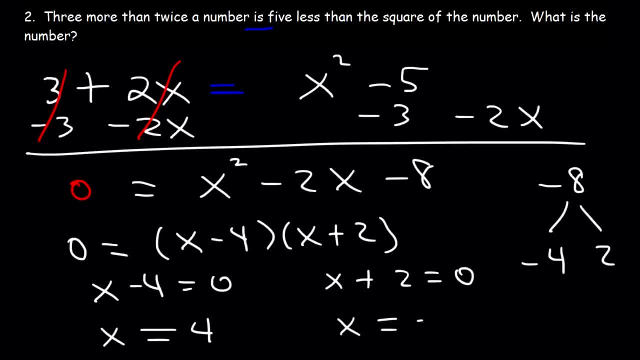 If we subtract both sides by 2, x is equal to negative 2. So the number has two possible values: It can be 4 or negative 2.. Now, if the question specified that it was a positive number, we would choose 4.. 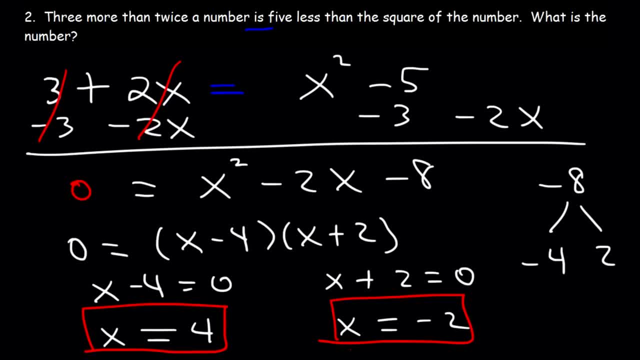 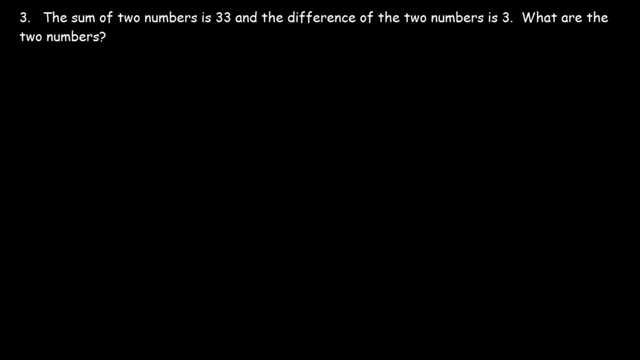 If it mentioned that it was a negative number, we would choose negative 2.. But it didn't really specify the sign of the number, so both answers are possible in this problem. Here's another problem that you could try. The sum of two numbers is 33, and the difference of the two numbers is 3.. 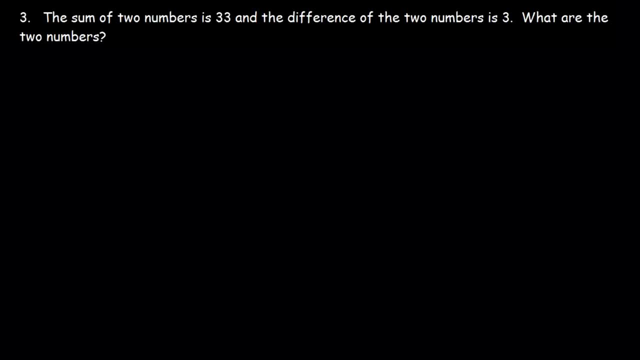 What are the two numbers equal to? The sum of two numbers is 33, and the difference of the two numbers is 3.. What are the two numbers equal to? If you're dealing with two numbers, you need two variables. The first variable, let's call it x. 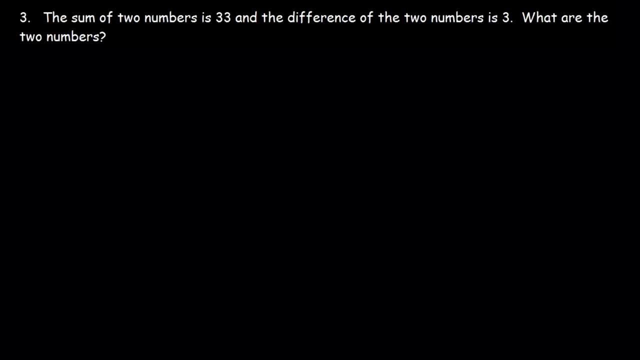 The second one, y. So the sum of two numbers, that is, x plus y, is, which means equals 33.. The difference of the two numbers, that's x minus y, is 3.. So we have two equations and two variables. 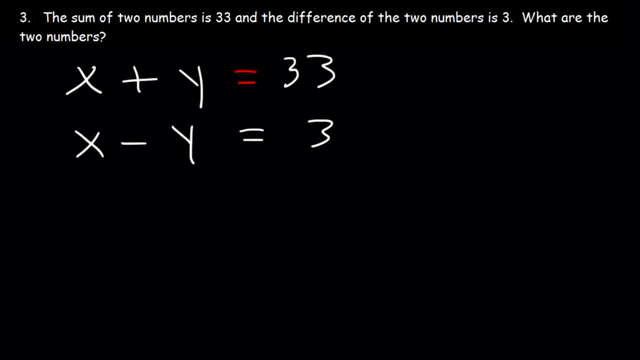 How can we find the two numbers? How can we find the two numbers? So we need to solve it as a system of equations. We can use the substitution method or the elimination method, also known as the addition method. Let's use the elimination method. 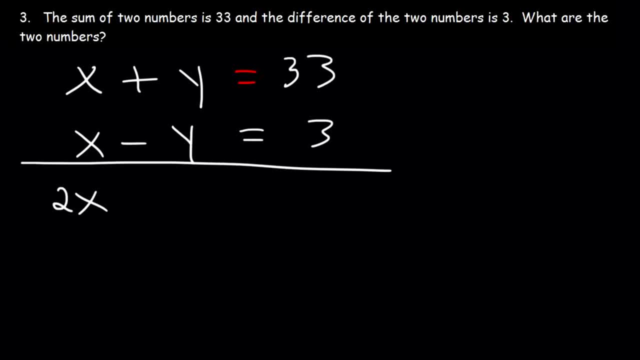 If we add the two equations x plus x is 2x, y plus negative y cancels, they add up to 0.. 33 plus 3 is 36, so 2x is equal to 36.. Therefore x is 36 divided by 2, or 18.. 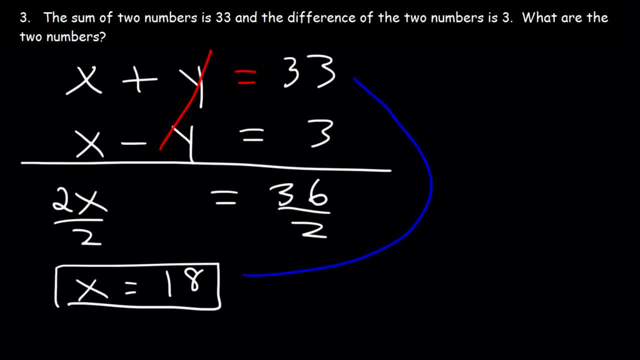 Now that we have the value of x, we can plug it into this equation to find y. So 18 plus y is equal to 33, so all we have to do is subtract both sides by 18.. 33 minus 18 is 15, and so that's the second value. 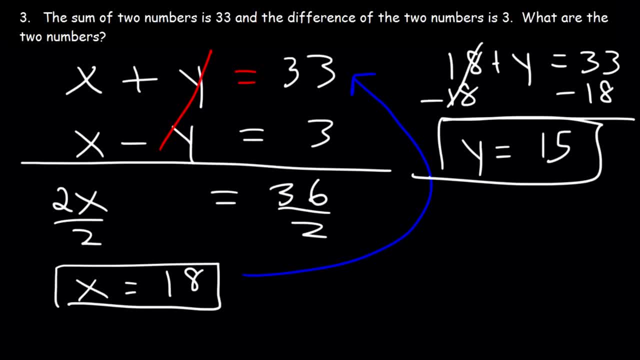 The sum of the two numbers 15 plus 18, is 33.. The difference of the two numbers is that the sum of the two numbers 15 plus 18, is 3.. So therefore, these are the two numbers. 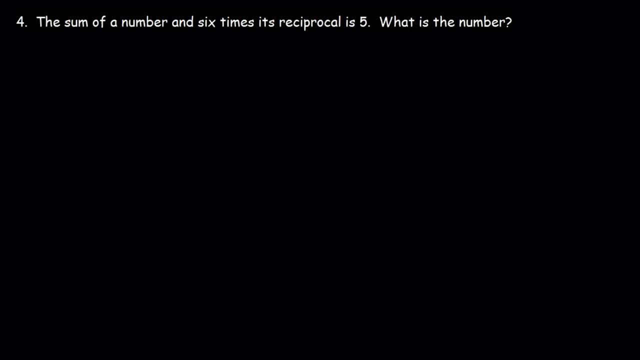 Number 4.. The sum of a number and 6 times its reciprocal is 5.. What is the number? So we're dealing with the sum, which is addition. The number is x and we're going to add it to 6 times its reciprocal. 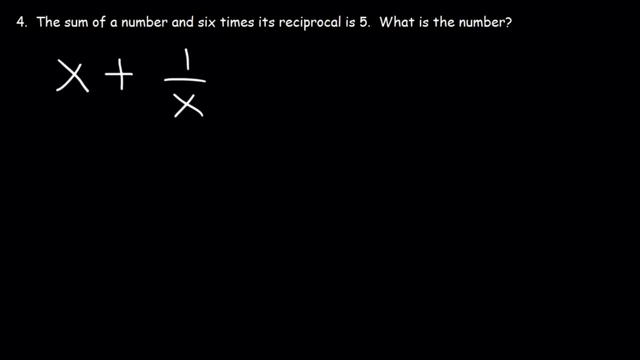 The reciprocal of x is 1.. So the sum of x is 1 over x, So 6 times its reciprocal is 1 over x times 6, which is the same as 6 divided by x. And all of that, the sum of those two things is 5, or equals 5.. 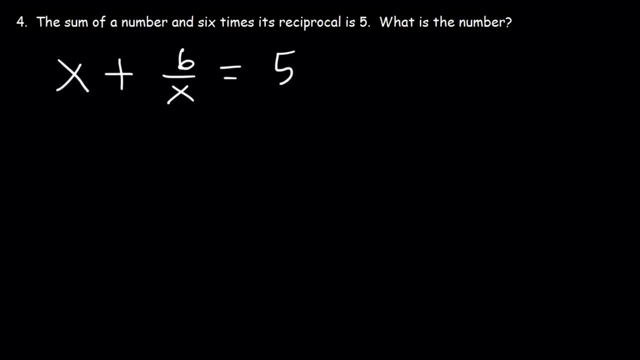 What is the number? The best way to solve this particular problem is to get rid of the fraction. You can do that by multiplying both sides by the denominator. So the number is x. So x times x is x squared. If we multiply 6 divided by x times x, these will cancel and it's just equal to 6.. 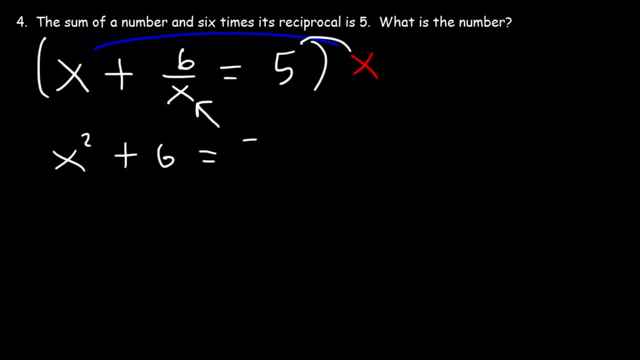 So this is going to be plus 6. And then 5 times x is 5x. Now let's subtract both sides by 5x. So x squared minus 5x plus 6.. So x squared minus 5x plus 6.. 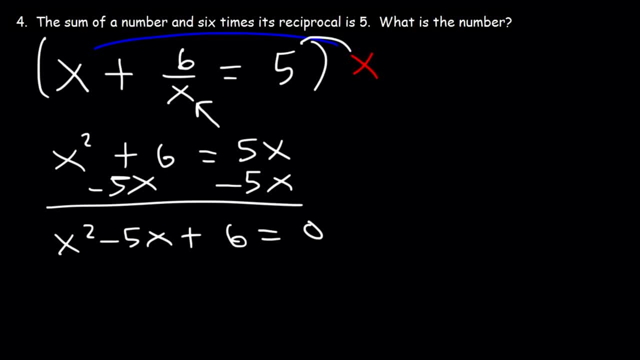 So x squared minus 5x plus 6 is equal to 0.. So we have a trinomial or a quadratic expression. Let's factor it. What two numbers multiply to 6, but add to the middle coefficient negative 5?? 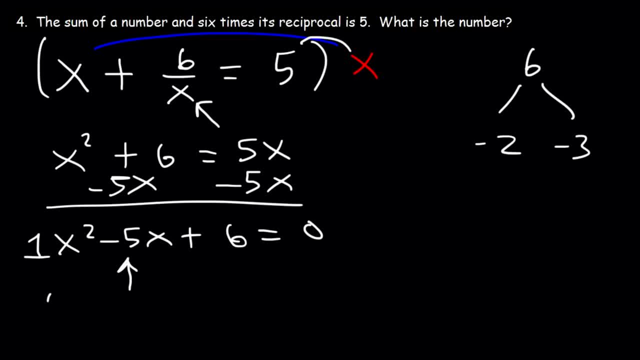 This is going to be negative 2 and negative 3.. So to factor it, it's x minus 2 times x minus 3.. So we're going to set the two factors equal to 0, and solve. So x is equal to positive 2 and positive 3.. 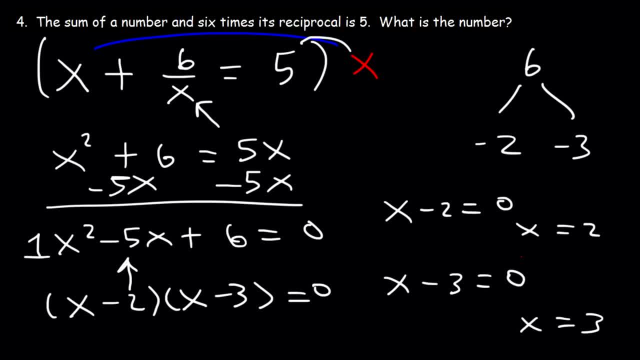 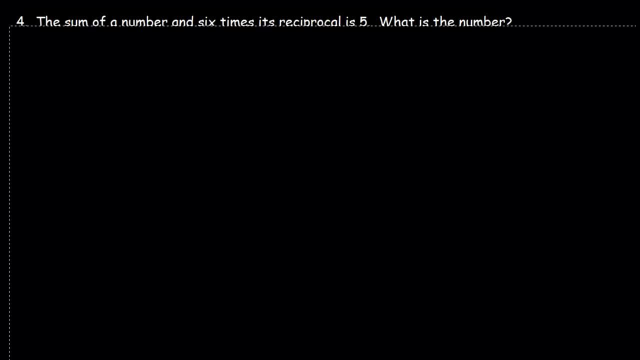 So x is equal to positive 2 and positive 3.. So now let's check it and let's make sure that it's correct. Let's try 2.. So the sum of the number 2 and 6 times its reciprocal, that 6 divided by 2, is 5.. 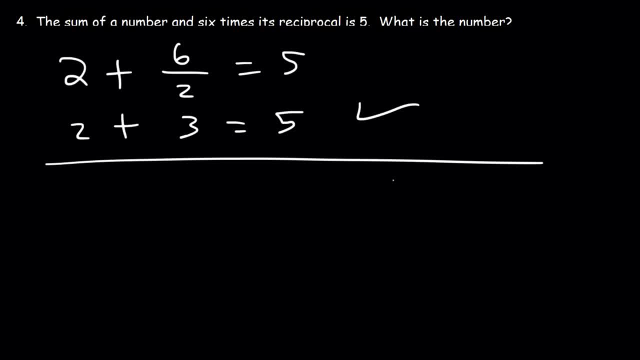 Six divided by 2 is 3,. 2 plus 3 is 5.. Now let's say the number is 3.. The reciprocal is 1 over 3 times 6.. Let's see if that's 5.. 5 times 2 is x plus 3,. 6 times 1 is x. 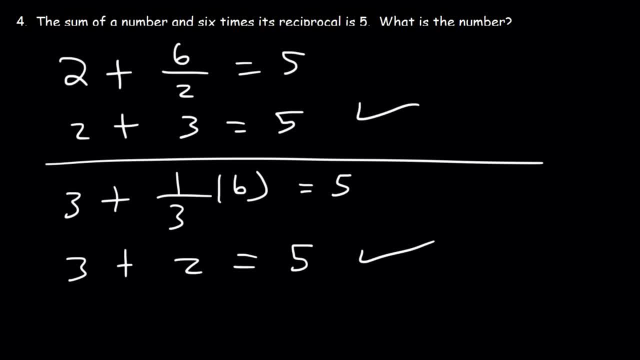 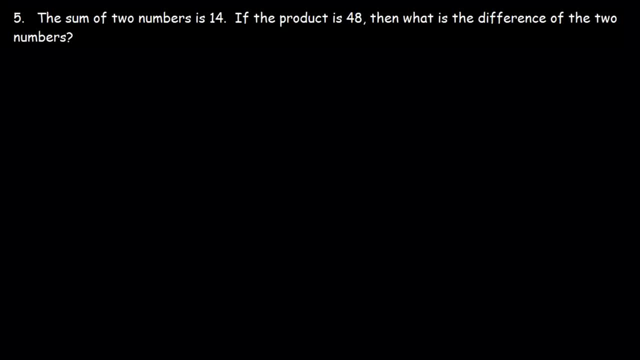 divided by 3 is 2.. 3 plus 2 is 5.. So the number can be 2 or 3.. Number 5,, the sum of two numbers, is 14.. If the product is 48,, then what is the difference of the? 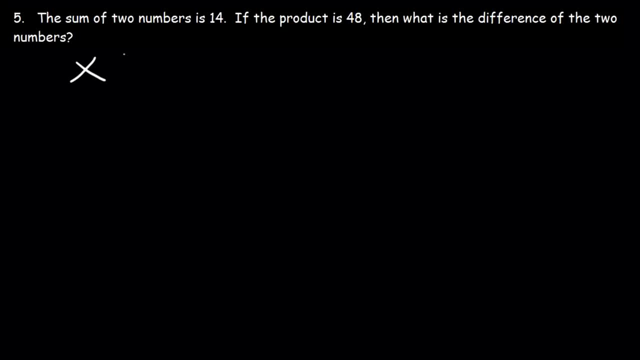 two numbers, So x plus y. the sum of two numbers is, or equals 14.. The product which is x times y, that's 48. So our goal is to find the value of x and y. Then we could find the difference of the two numbers. So what do we need to do For? 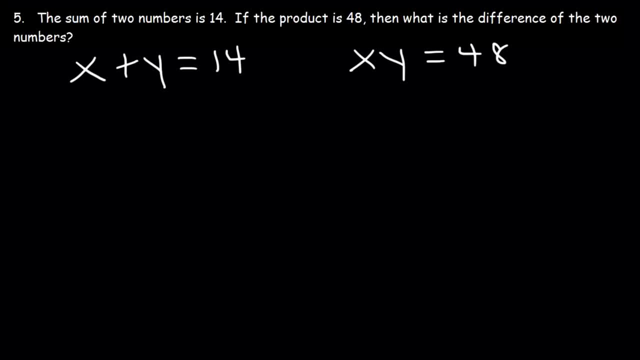 this particular problem, the best way to find the answer is to use the substitution method as opposed to the elimination method, since we have two equations and two variables. So, in the first equation, let's subtract both sides by x. Let's subtract both sides by x. 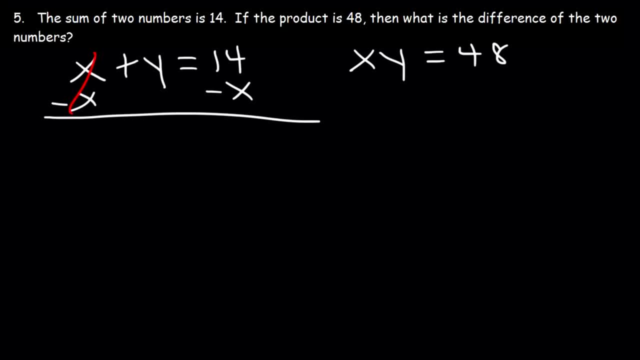 Let's get y by itself. So therefore, y is equal to 14 minus x. Now what we're going to do is we're going to replace this y with 14 minus x, So we can get one equation with one variable. Therefore, x times 14 minus x is 48.. Let's distribute x to 14. 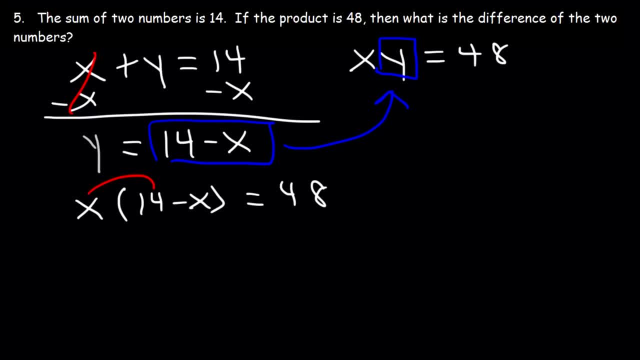 minus x, So x times 14, that's 14x x times negative. x is negative, x squared and that's equal to 48.. So everything on the left side, let's move it to the right side so that x squared can be. 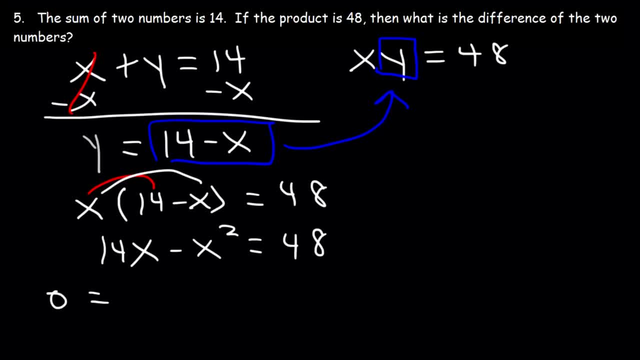 positive. So if x squared is negative on the left side, it's going to be positive on the right side, And if 14x is positive on the left side, it's negative on the right side. So we have another trinomial and let's see if we can factor it. 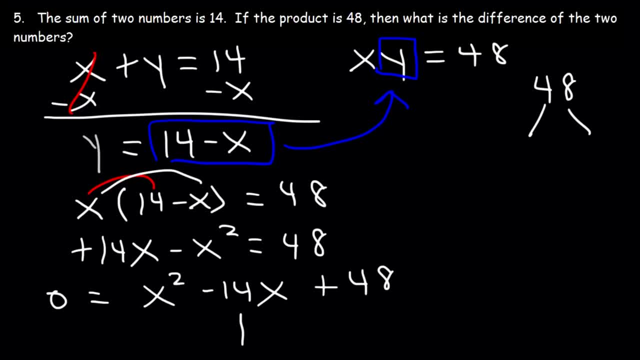 What two numbers multiply to 48 but add to the middle coefficient negative 14? Eight times six is 48, and it adds to 14, but we need to use negative eight and negative six because we want it to add to negative 14.. So to factor this expression, it's going. 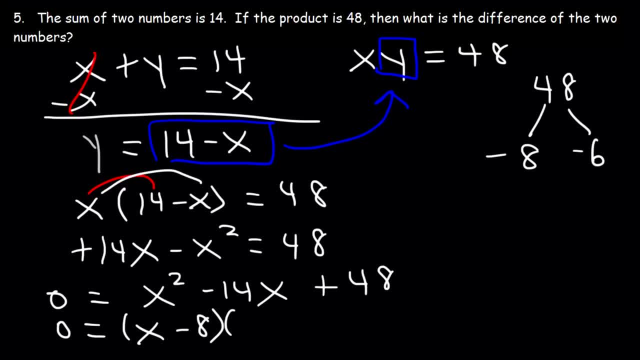 to be x minus eight times x minus six, And we need to set each factor equal to zero. So if x minus six is equal to zero and if we add six to both sides, x is equal to positive six. And then if we set the other factor equal to zero and add eight to both sides, x is 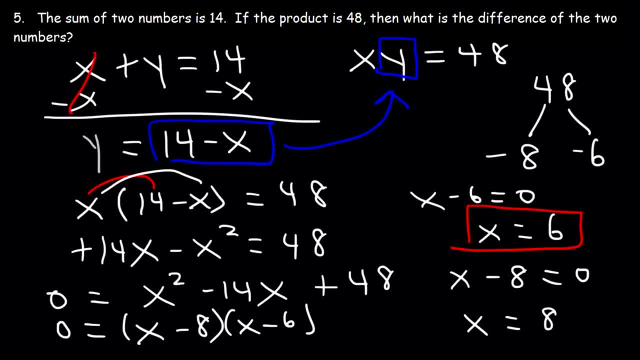 equal to positive eight. So those are the two possible values of x. Now what about y? So let's use this equation now: y is 14 minus x. So when x is six, y is going to be 14 minus six, which is eight. So when? 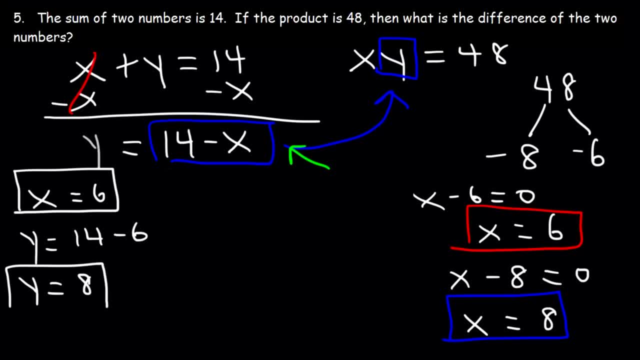 x is six, y is eight. Now what about when x is eight? 14 minus eight is six, So y is six when x is eight. In either case, the two numbers are six and eight. Six and eight adds up to 14, and six times eight will give us a negative six. 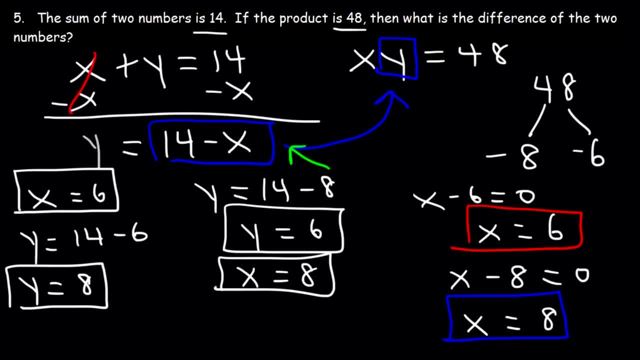 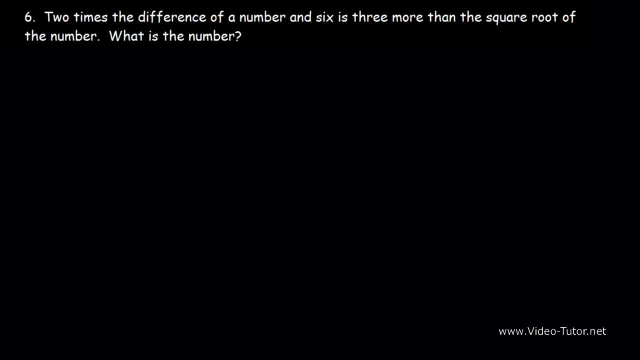 So that's a product of 48.. Now our goal is to find the difference of the two numbers, That is, eight minus six. These two numbers differ by two. They're two units apart on the number line. So this is the answer. The answer is two Number six, Two times the difference. 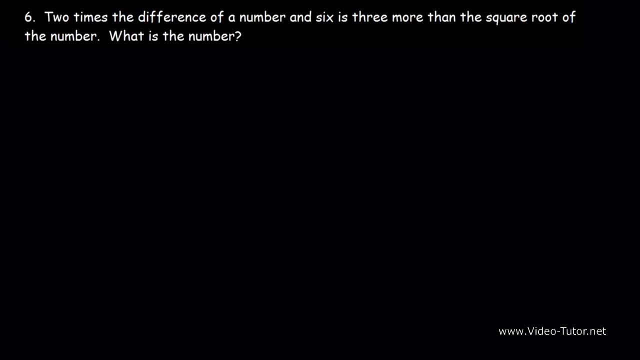 of a number, and six is three more than the square root of the number. What is the number? So first we have the difference of a number and six, So that's going to be x minus six or six minus x. And then it's two times that difference and that's going to be three more than. 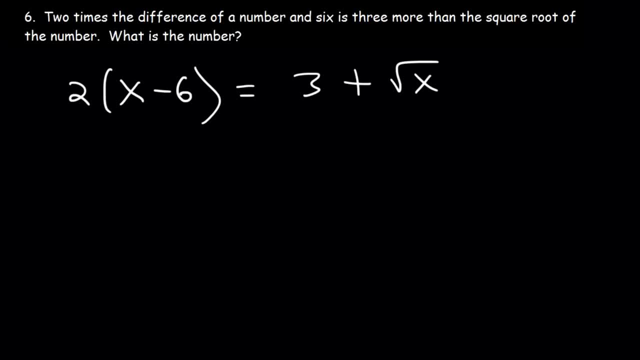 the square root of x. What is the number? So what do we need to do in this problem? Whenever you have a radical or square root, you want to square both sides, but you need to get this by itself. So first let's distribute 2 to x minus x. 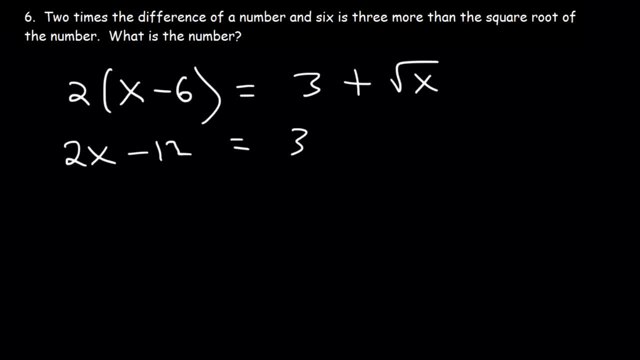 So it's 2x minus 12. That's equal to 3 plus root x. And then let's subtract both sides by 3. So 2x minus 15 is equal to the square root of x. At this point you want to take the square of both sides. 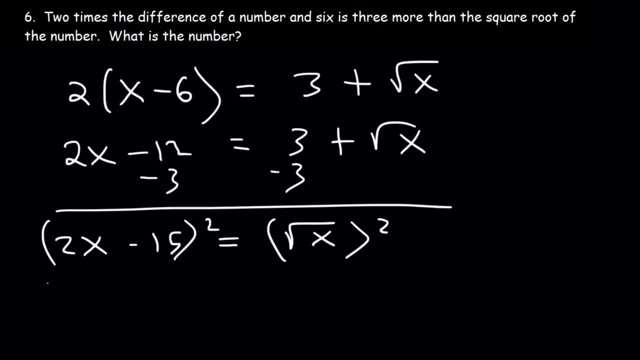 2x minus 15 squared is basically 2x minus 15 times 2x minus 15.. On the right side, the square of the square root of x is x. Radical x times radical x is the square root of x squared, which is just x. 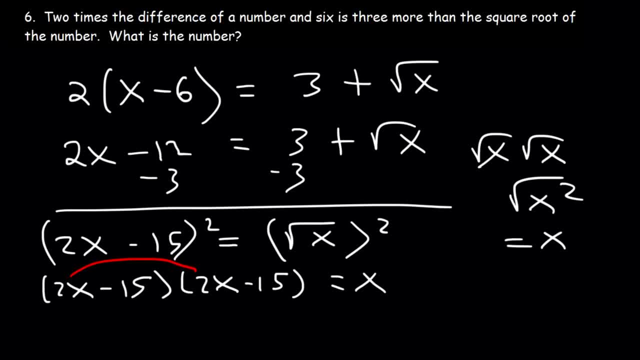 Now we need to FOIL 2x minus 15 times 2x. 2x times 2x is 4x squared, And then 2x times negative 15, that's negative 30x, and this is another negative 30x. 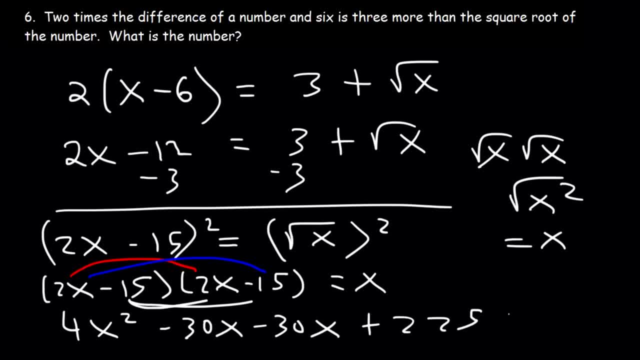 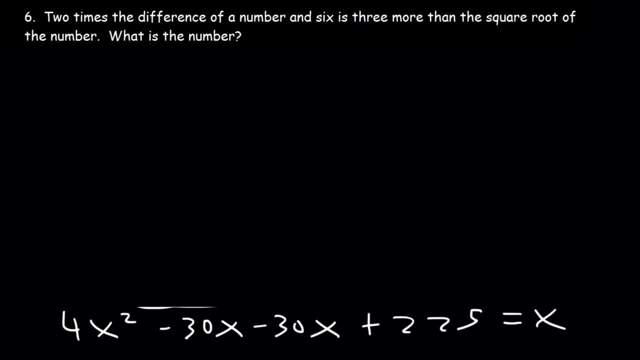 Negative 15 times negative 15, that's 225.. And that's equal to x. So now let's combine like terms: Negative 30x minus 30x is negative 60x. Okay, So all of this is equal to x. 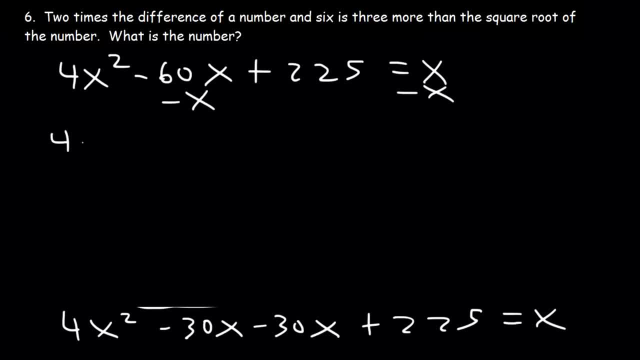 Now, if we subtract both sides by x, 4x, squared minus 61x plus 225 is equal to 0.. So we can try to factor this expression or we can use the quadratic formula. Let's see if we can factor it. 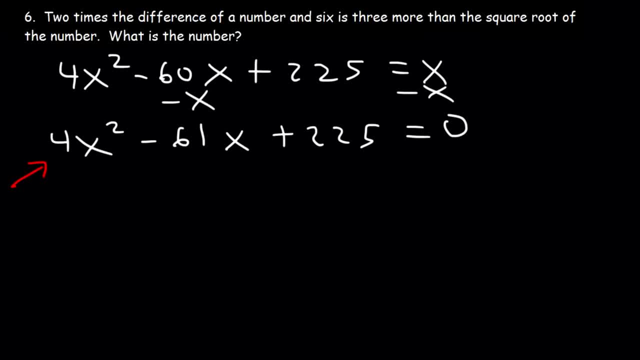 Now, this time we have a trinomial where the leading coefficient is not 1,, it's a 4.. Okay, So we've got to multiply 4 and 225.. 4 times 225 is 900.. 4 times 200 is 800. 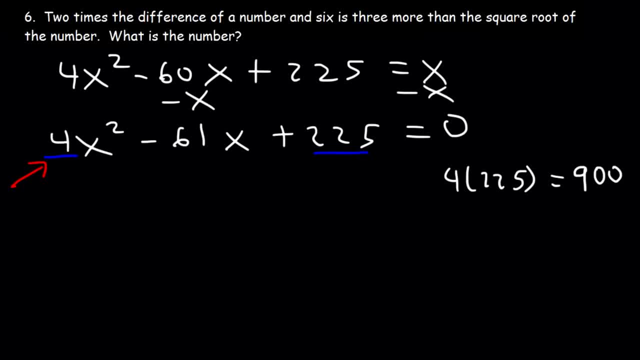 And 4 times 25 is 100.. 800 plus 100 is 900.. Now what two numbers multiply to 900, but also add to 61?. So it might be good to use a calculator at this point, Or what you could do. 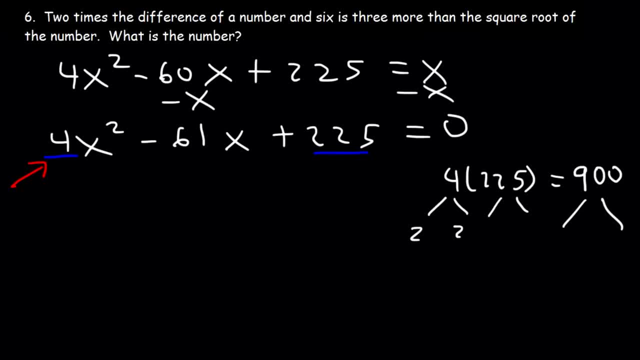 Is: break down 4 into 2 and 2, and 225 into 15 and 15.. So this can tell you numbers that go into 900.. For example, 15 is a factor of 900.. The remaining terms are 2 times 2 times 15, which is 60. 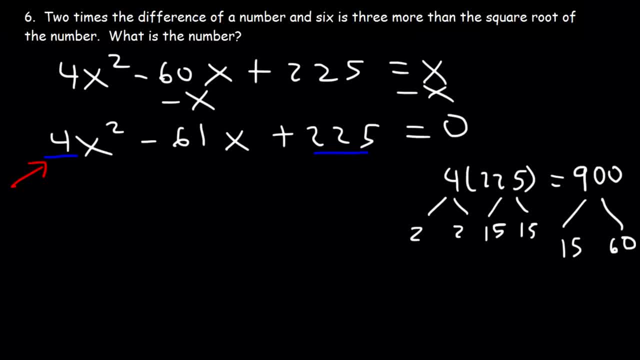 So 60 times 15 is 900.. But these two numbers, they both have to be negative And they don't add up to negative 61. Okay, So we need to change it. Factors of 15 are 5 and 3.. 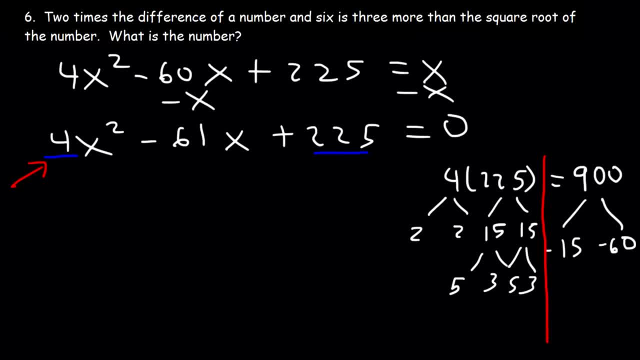 Let me just draw a line and separate these two numbers, So we can use 5 and let's say 5 and 5. That's 25.. And then the numbers that are left over are 3. And 5.. 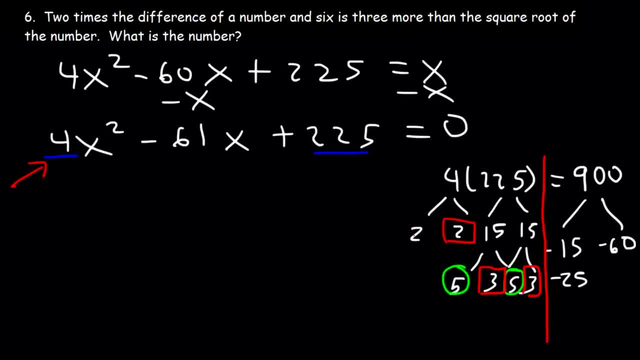 So it'll only add up to 9.. So if we subtract the 1., And then we subtract the 2. And then we subtract the x And the às, And now we're all squared by 8. And I wanna get these numbers higher than 9.. 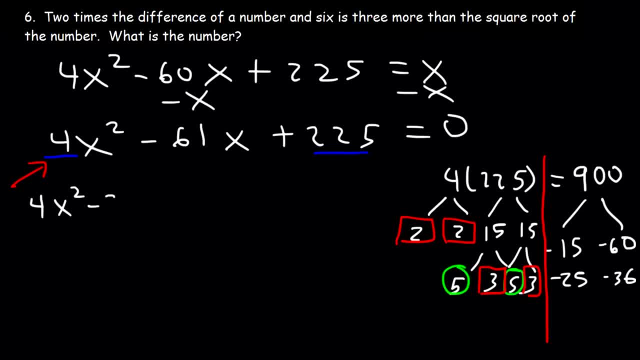 Let's break down these numbers. And now that's subtracted. And then what we're gonna do is we're gonna add 3. Let's subtract that and 8. I chose to put the 25x next to 225 because you can clearly see that both numbers are. 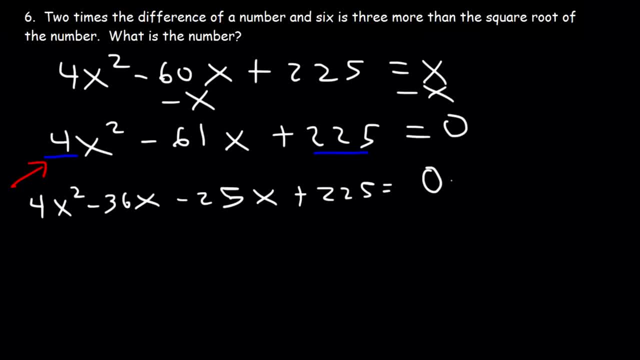 divisible by 25.. Our next step is to factor by grouping. In the first two terms we need to take out the GCF, the greatest common factor, which is 4x. 4x squared divided by 4x is x. 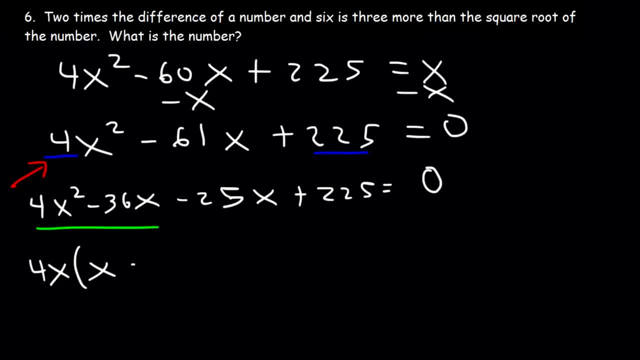 Negative 36x divided by 4x is negative 9.. On the last two terms, we need to take out negative 25.. Negative 25x divided by negative 25 is simply x 225 divided by negative 25 is negative 9.. 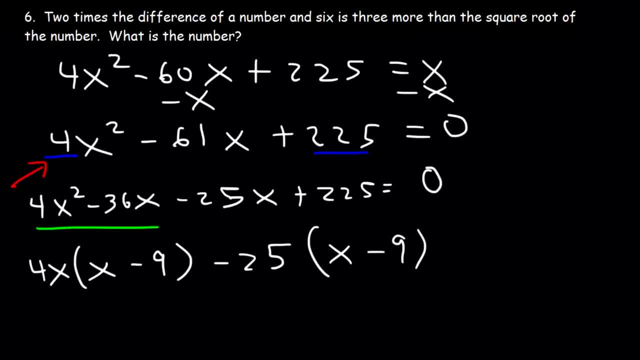 If you have 9 quarters, you have $2.25.. So 9 times 25 is $2.25.. At this point we can factor x minus 9, and we do so. we just have to write it once. 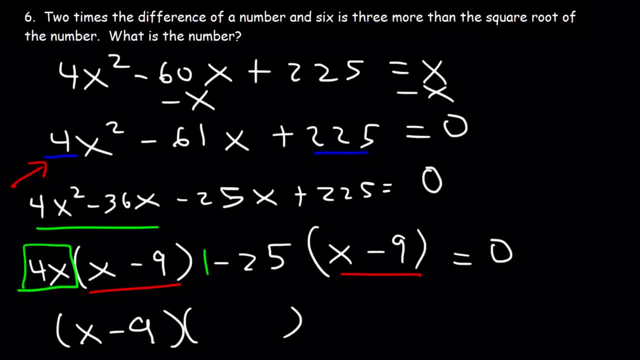 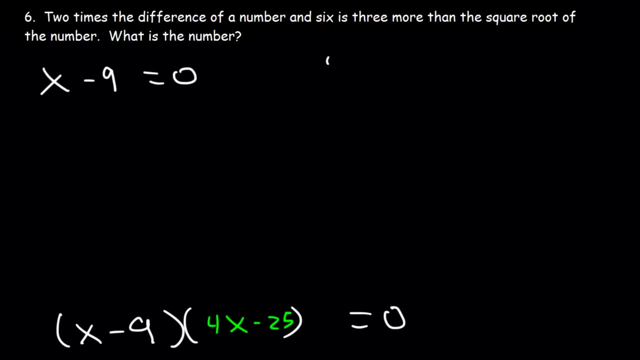 Now the stuff on the outside, the 4x and the negative 25, that's going to go in the second parentheses. So this is what we have. So we can set x minus 9 equal to 0. And 4x minus 25.. 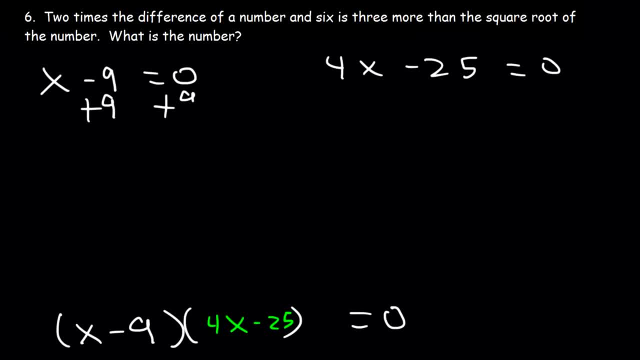 5 equals to 0. So on the left we're going to add 9, on both sides, So x is equal to 9.. On the right side, we'll add 25.. So 4x is equal to 25.. 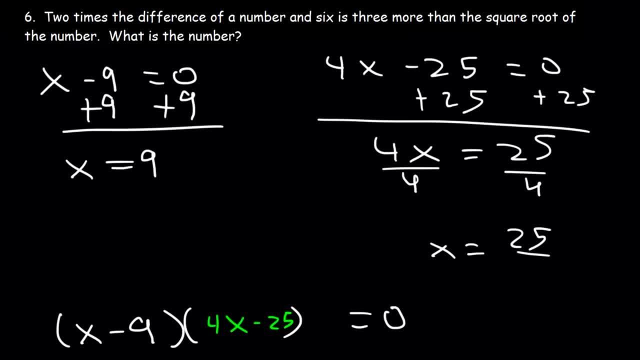 And if we divide by 4, x is 25 over 4.. So the number could be 9 or 25 over 4.. But let's see which one is correct, Because when dealing with radicals you may have an extraneous solution. 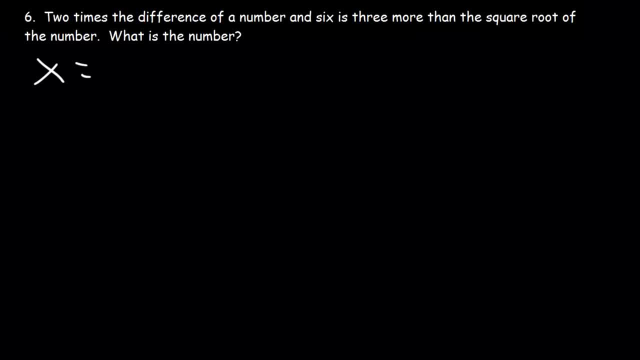 So the number could be 9 or 25 over 4.. But let's see which one is correct, Because when dealing with radicals, you may have an extraneous solution. But let's see which one is correct. Now, before we check it, let's convert 25 over 4 into a decimal value. 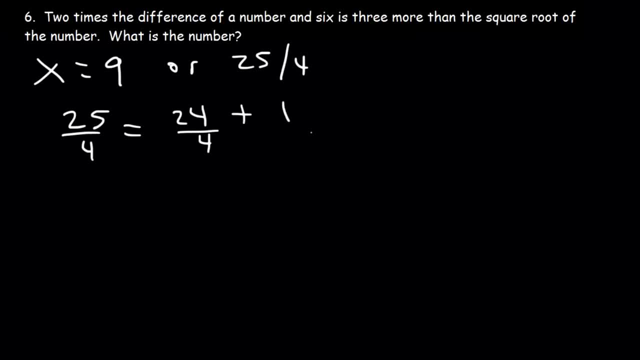 25 is 24 plus 1.. 24 divided by 4 is 6., And one fourth is 0.20.. So therefore, this is 6.25.. 0.25. was 2x minus 6, which is equal to the square root of x plus 3.. 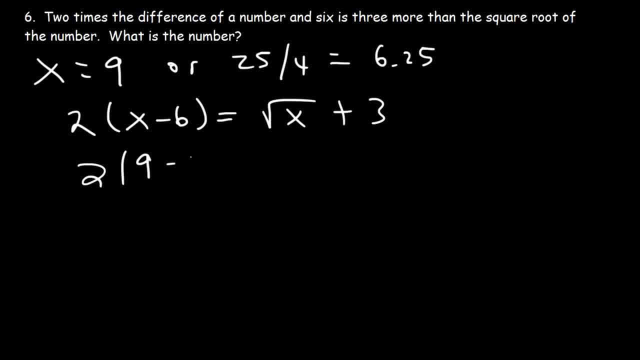 So let's try 9.. So 2 times 9 minus 6, is that equal to the square root of 9 plus 3?? 9 minus 6 is 3.. The square root of 9 is 3.. 2 times 3 is 6.. 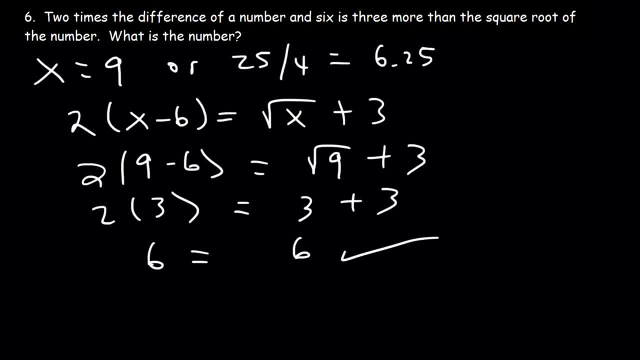 3 plus 3 is 6, so that works. Now let's make sure that the other one works as well too. So let's plug in 6.25.. 6.25 minus 6 is 0.25.. And the square root of 6.25 is 2.5.. 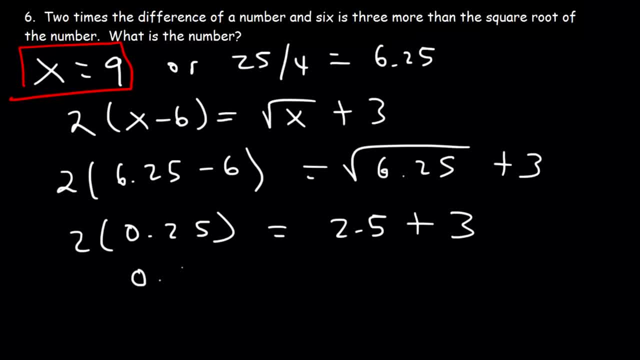 2 times 0.25 is 0.5.. And 2.5 plus 3 is 5.5.. So there's a mismatch. So therefore this answer doesn't work. x is equal to 9 if we write the equation like this: